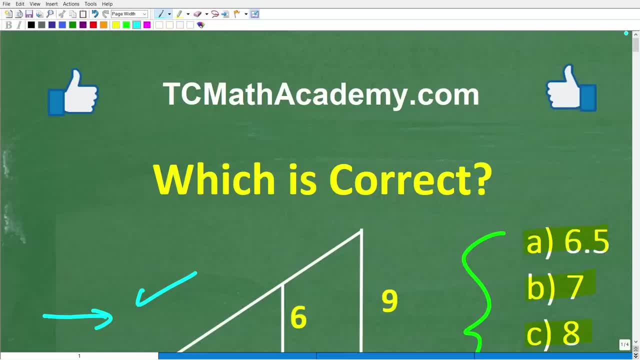 have been teaching middle and high school math for decades and if you need help learning math, check out my math help program at tcmathacademycom. You can find a link to that in the description below, and if this video helps you out or if you 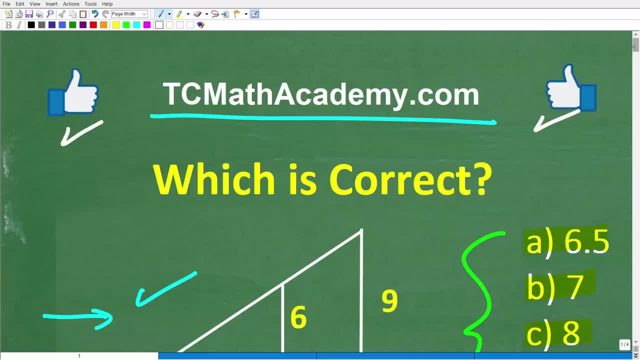 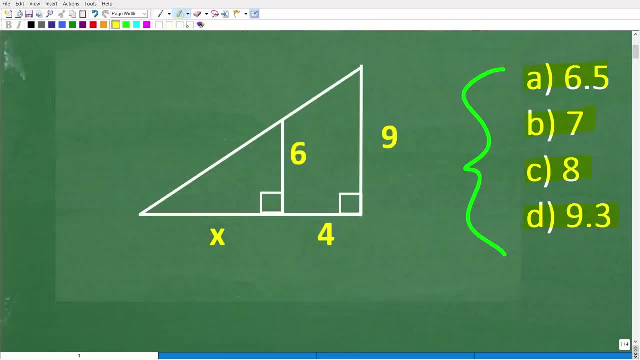 just enjoy this content. Make sure to like and subscribe, as that definitely helps me out. All right, Now, once again, here is our situation. We have these two triangles and we want to take note of what type of triangles we're dealing with. Now hopefully you're saying, oh, I know what type. 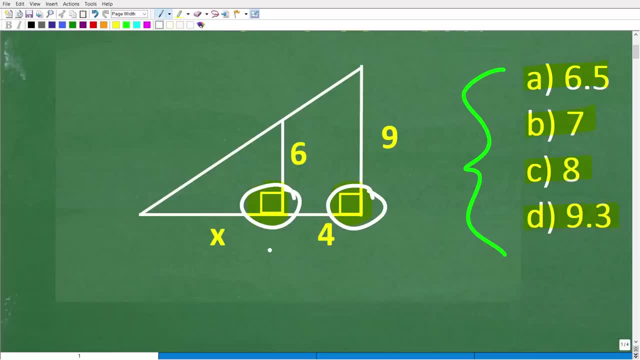 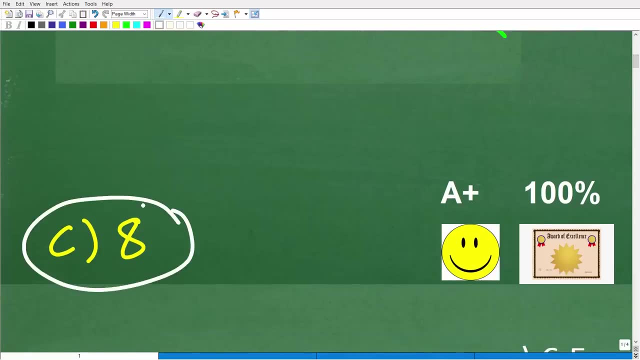 of triangles. these are Mr YouTube Math Man. Well, that is fantastic. Now let's take a look at the answer. Then, of course, we'll get into the solution. But the correct answer here is C, which is A. All right Now, if you got this right, you definitely get a happy face, an A+. 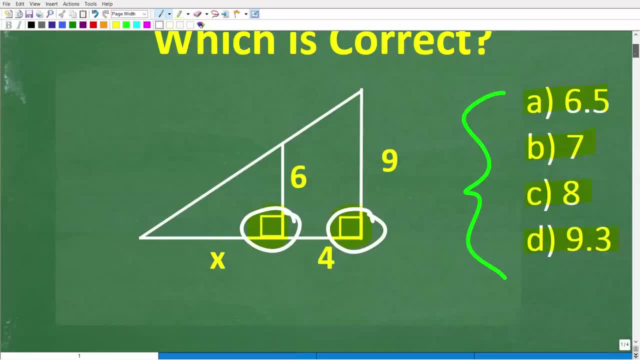 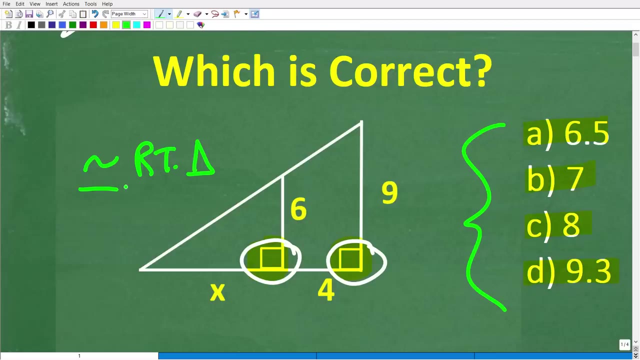 a 100% and a certificate of excellence, because you appear to be a certified professional expert in the area of similar right triangles. All right, Now this is a big topic that you study in geometry, And if you never heard of similarity, well, this is going to be a nice kind of. 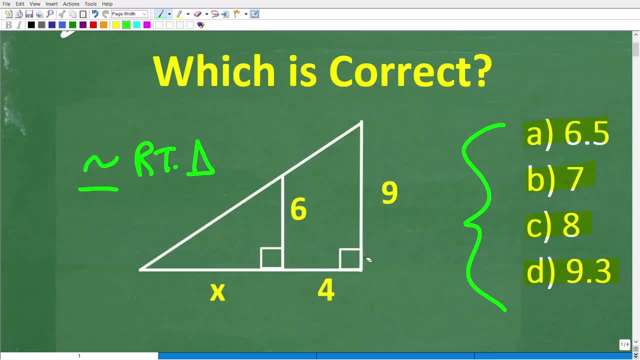 introduction to the concept. It's not that difficult, But in kind of a real basic sense similarity is. effectively, if we look at this triangle and this triangle, they appear to be basically the same triangle, just that the bigger triangle is like a zoomed. 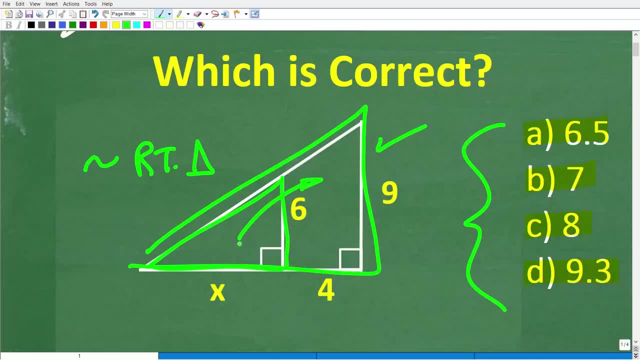 out version or an expanded version of the smaller triangle. Well, this concept of basically the same shape but different sizes- So if I have this box and here is kind of a larger version of it but we have the same angles and all the sides are in proportion- Well, this concept is called. 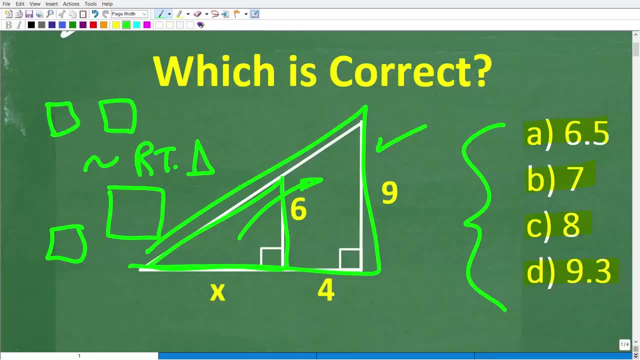 similarity Versus the concept of having exactly two figures that are exactly the same size, shape and everything else That's called congruent, All right. So that's what we're dealing with in this particular problem, And this is not that difficult. But let's go ahead and take. 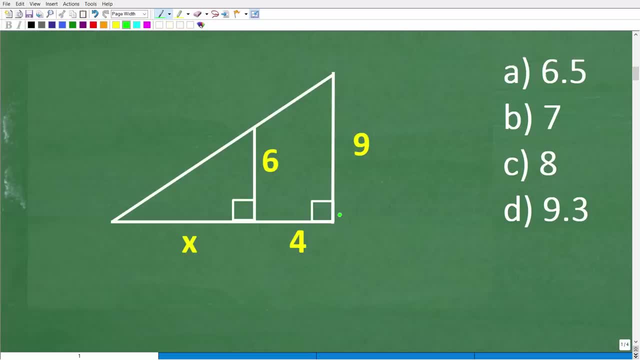 a look at the problem here. And we're dealing with right triangles, right? So some of you might be saying, oh, Mr YouTube, Math Man, I know a lot about right triangles And that's wonderful. You're like. I'm going to start thinking about the Pythagorean theorem: A squared plus B squared. 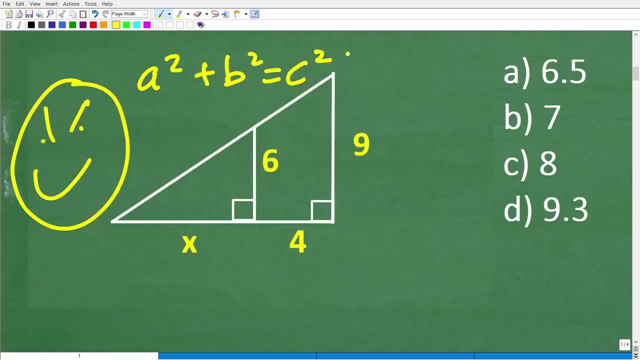 Is equal to C squared, And that would be fantastic, But we really don't have enough information to use the Pythagorean theorem to figure out this problem, because A squared plus B squared is equal to C squared, In fact. let me write this up here again: This is basically the relationship between the. 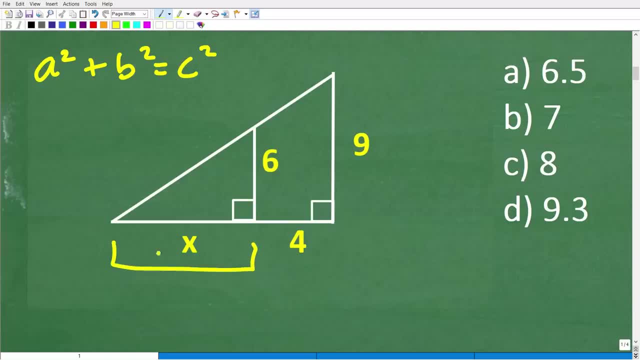 sides of a right triangle. So let's suppose this side right here of this triangle was I don't know. let's say four and this side was three. We can figure out the longest side, which is the, by using the Pythagorean Theorem. So basically, C is always the longest side of a right triangle. 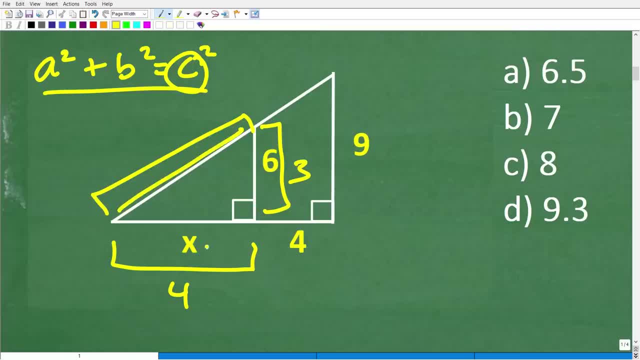 that's called the hypotenuse. So we could solve for this by just plugging these numbers in, So this would be: 3 squared plus 4 squared is equal to C squared. So we get: 9 plus 16 is equal to C. 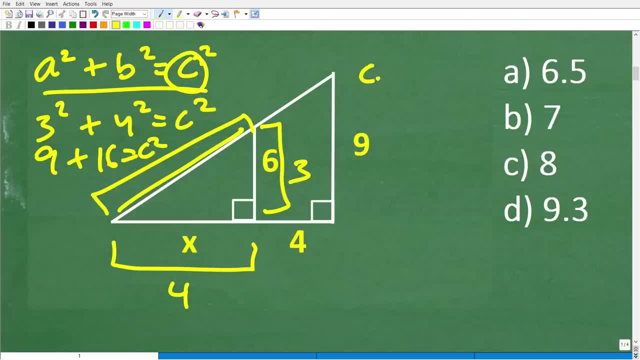 squared. I'm kind of sloppy here trying to squeeze this in, but we have C: squared is equal to 25.. We take the square root of both sides, we get C is equal to positive negative 5, but we're talking about distance here, so C is equal to 5.. So that would be the the length of this side of this. 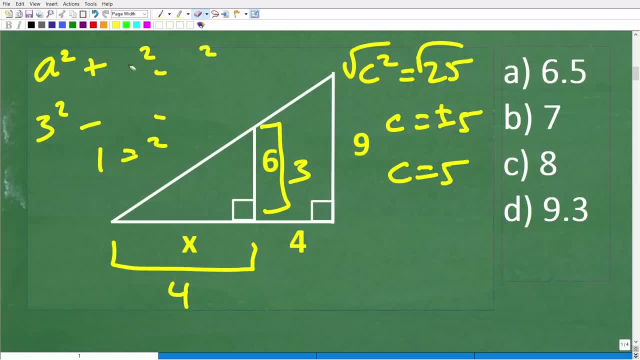 right triangle, the hypotenuse. But in order to solve a right triangle problem with the Pythagorean Theorem, you need two out of the three sides. Okay, so here what we're looking at is: we don't have this information, and we don't have this information, we only have this side. 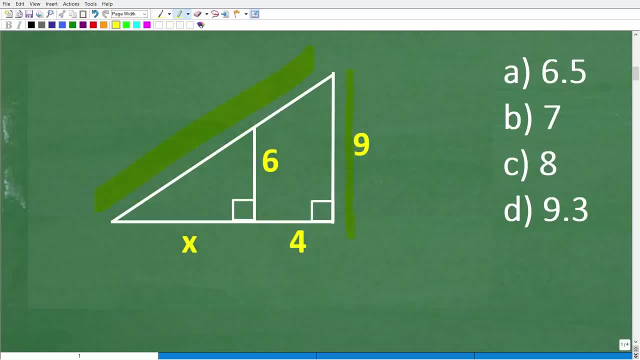 And if you look at the big triangle, we have this side, but we don't have the hypotenuse and we don't have this side as well. So what are we supposed to do? Well, some of you might be saying: I know what I'm going to do, Mr YouTube Math Man, I'm just going to take a guess. Well, that's exactly what. 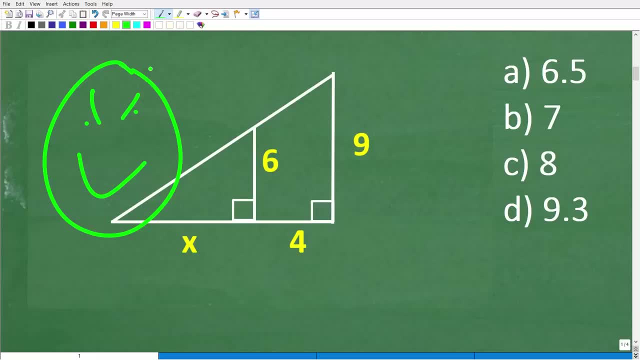 you should do So. let's just look at the problem and you know you kind of think about it. you know if you're saying, ah, this, this is, this is 6 and this side looks longer than 6.. I don't know, maybe this is like 7, or maybe this is 9.3.. 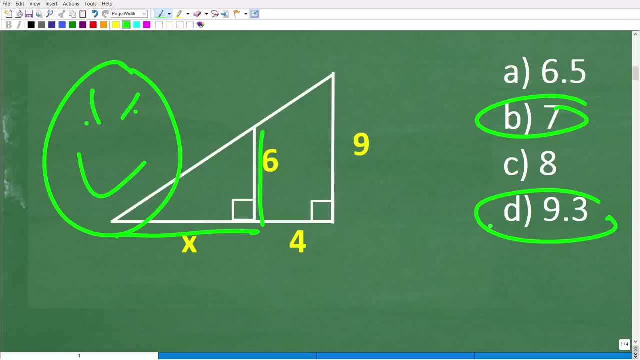 Thinking in those terms. I think that's excellent. so you know, obviously you want to take a guess, but these are wrong and the correct answer is 8.. So the only way to really figure this out is to actually know the math. Okay, so once again, we're dealing with this concept of similar right. 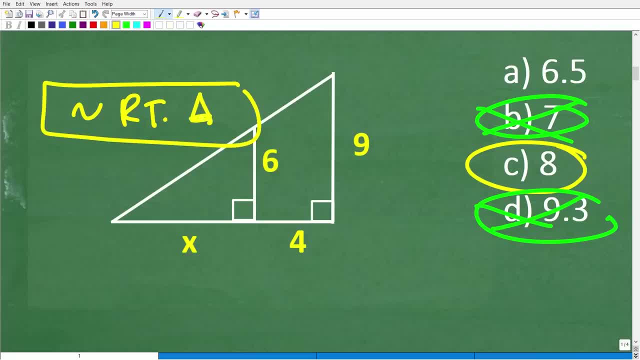 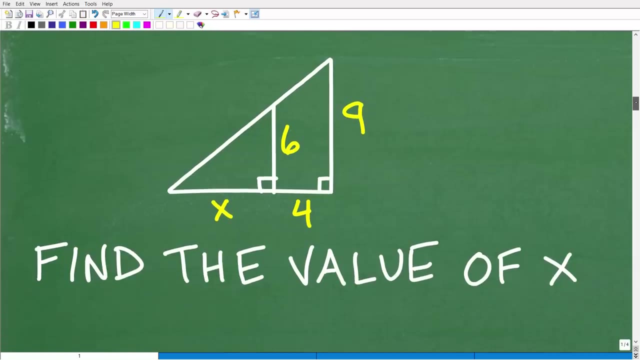 triangles, and this is a big topic in geometry, So I can't possibly teach you everything about similarity in this particular video, but I think you'll get the main concepts if you've never seen it before. Alright, so let's get into the solution right now. Okay, so here is our problem. we want to. 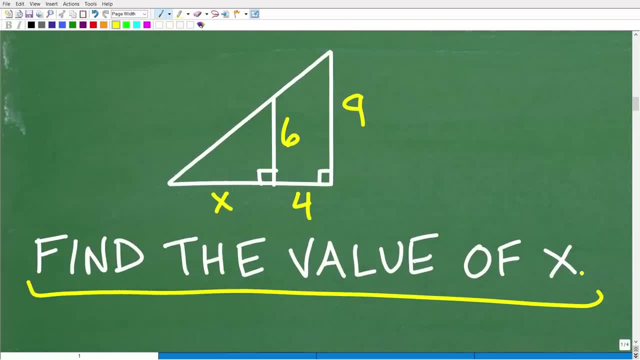 find the value of x? that's another way we could kind of phrase this question. Now, of course, I explained the problem because I didn't want anyone out there to be lost. but here is a triangle, we have a triangle in inside of the bigger triangle and they're both right triangles and we're looking 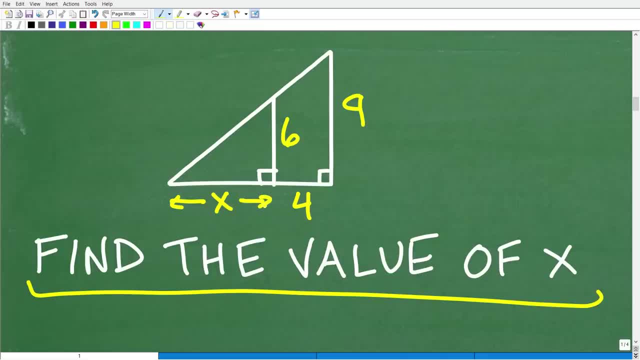 for this distance x. Okay, so what can we do? Well, we already discussed that we really can't use the theorem theorem, so we need another strategy, and that is going to be used. that is going to be using the concepts of similar right triangles or similarity. Okay, so, similar right triangles. 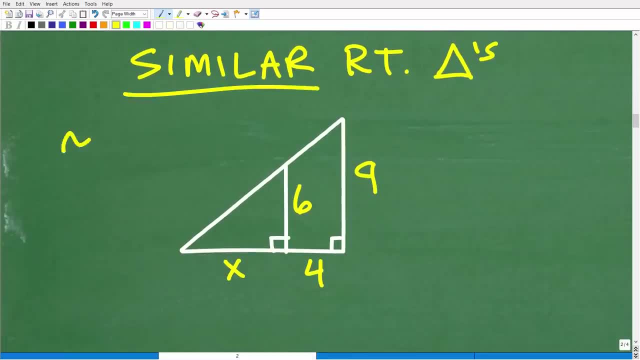 again, this concept of similarity is? well, here is the notation for it. So if I have this triangle and this triangle and they're similar to one another, you have this little squiggly line right here. Oftentimes this is the same. well, not oftentimes, you'll see this. 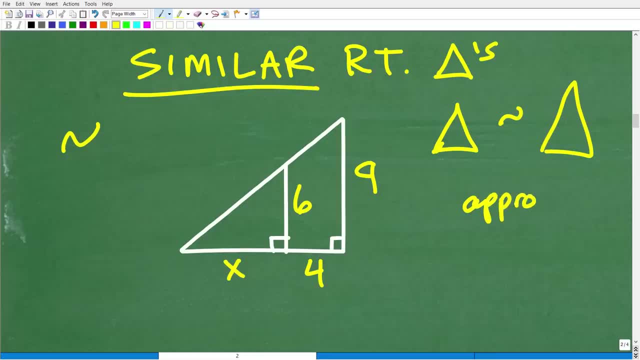 when we're trying to say something is approximately a particular value. so if something is approximately three in math, we could put that little squiggly line three. Okay, so this notation has various notations. it also, I believe, is not as well n-o-t but in geometry. when you see this, we're talking. 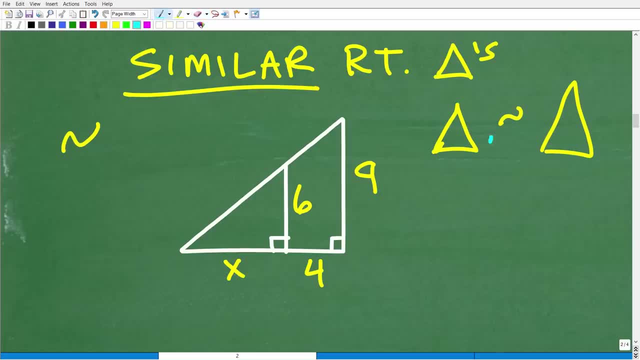 about similarity. and again, similarity is basically, if you take a figure and let's say you copy it, let's say you're on your computer and you're going to, just you know, select the copy it, A copy function, you paste it and then you expand this to make it larger or smaller. the larger: 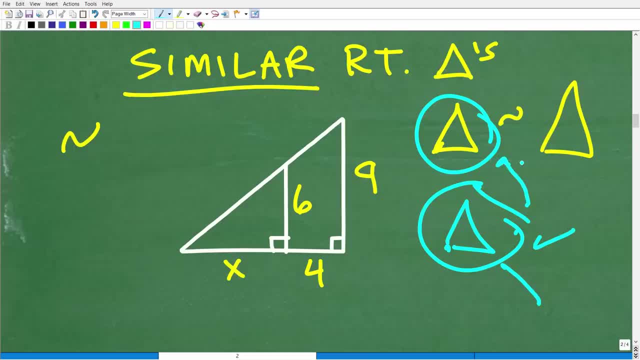 figure or the smaller figure as compared to the other figure. those two figures are similar, Okay, if you make an exact copy of it. so in other words, it's the same size and shape. that's congruent, right again, this is the notation for congruency. So congruency is a big topic in geometry, but so is 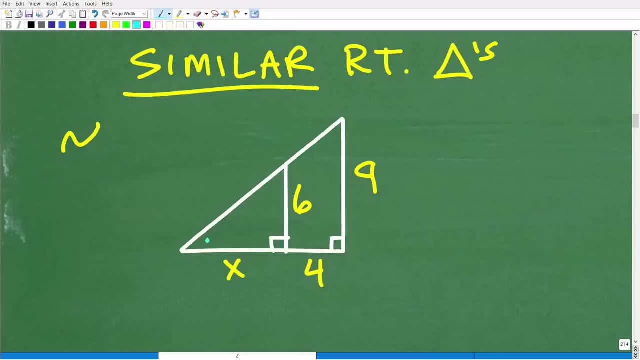 that I'm dealing with two similar right triangles. So basically, this triangle here and this triangle here are the exact same proportion, and that is the key idea when it comes to similar figures. right, basically the sides are in proportion, so you have the same angles. so I'm just kind of sketching this. 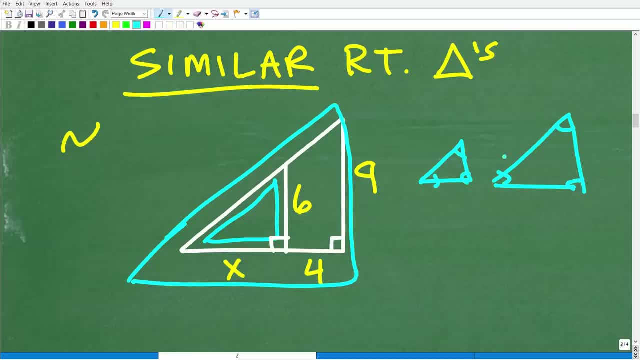 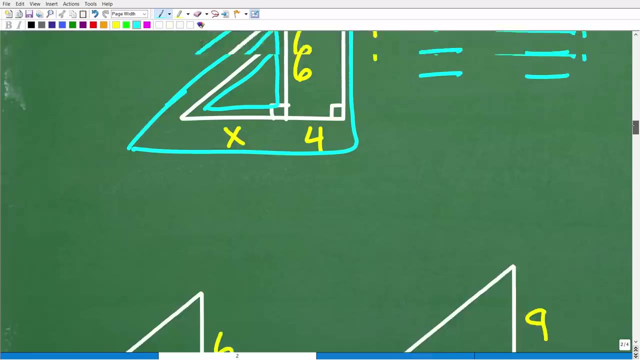 out this way. so here is our right angles. the angles are the same in similar figures, but the sides are in proportion. That is going to be the key in order for us to solve this problem. Okay, so let's go ahead and see how this is going to be set up. So what we want to do is actually break this problem up into two. 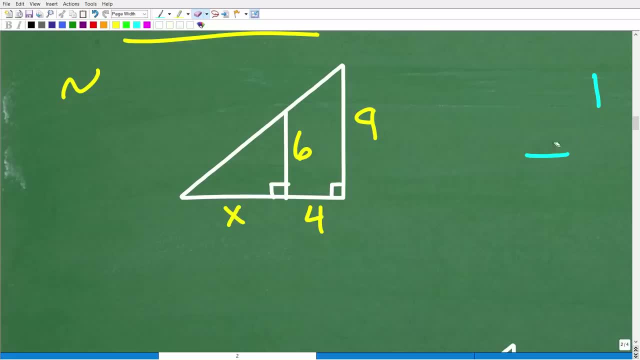 distinct triangles. Okay, so this is the kind of the strategy that you want to take. so some of you can actually see, oh, here's a separate triangle and here's the bigger triangle. but let's go ahead and just break this out. We'll draw this kind of, or sketch this out separately from the bigger triangle. 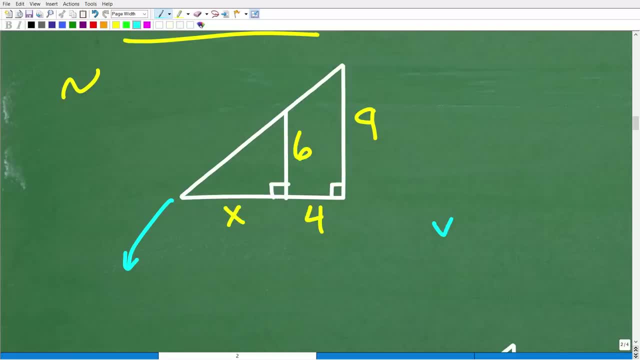 so we can see exactly what's going on Here between the sides. okay, so the smaller triangle is going to have six and X as its sides, and then the bigger triangle is going to have nine, and then what's this length going to be? well, that's going to. 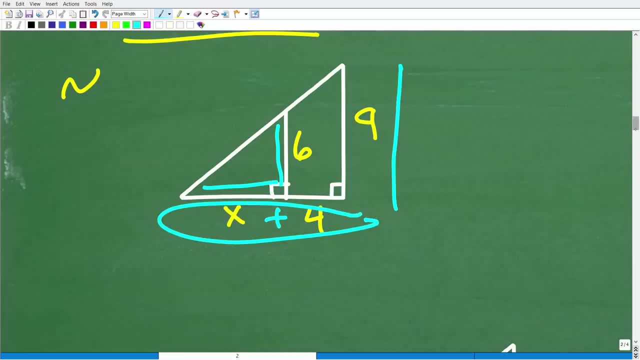 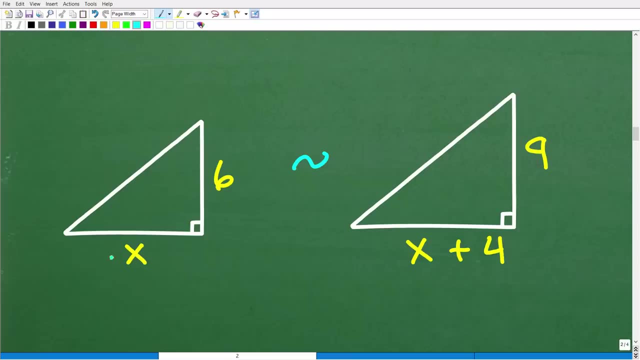 be X plus four. All right, so let's go ahead and take a look at that right now. so here is our two similar right triangles. All right, so the smaller triangle has six and X, and again we're looking for X plus four. Okay, so these sides are in proportion, in other words, the, the proportion from this side. 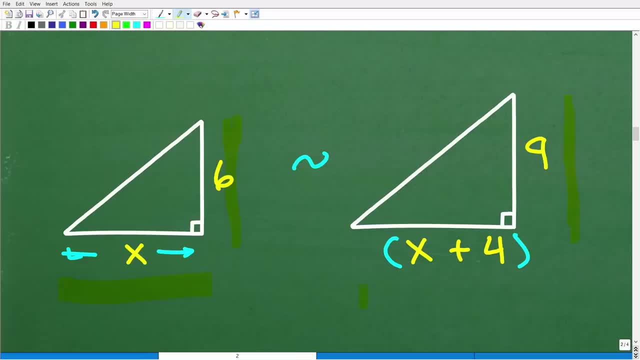 to this side is equal to the proportion of this and this, or the ratio between this length and this length, is the same thing as the ratio between this length and this length, meaning that these two ratios are in proportion. Okay, so hopefully you understand some basic math like how to set up and. 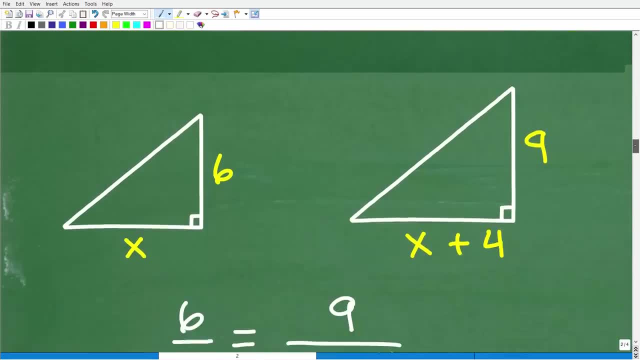 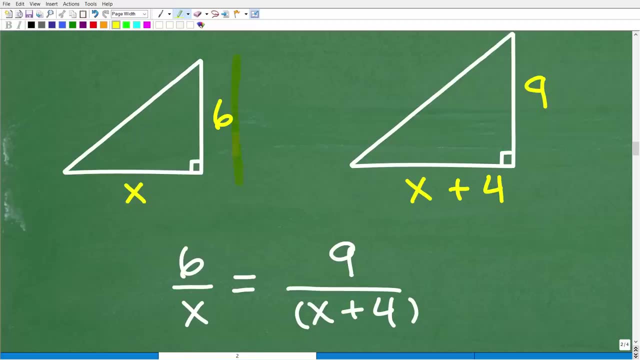 solve a proportion, and that's what we're going to do right now. So here is our two similar right triangles. so the height of the triangle, the proportion or the ratio of the height of the triangle. see, I have to kind of correct myself here and make sure that I'm using 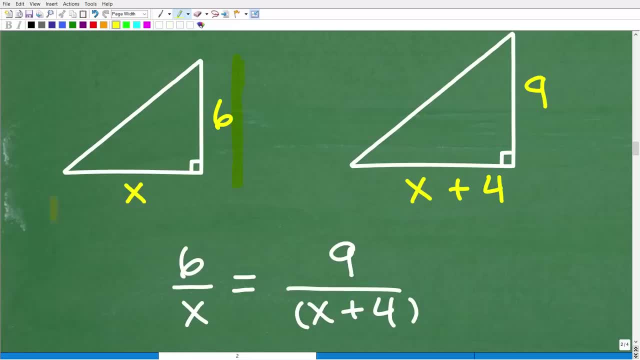 the correct term. so it's the ratio between the height and the. we'll call this the length. so the height to the length of the small triangle is going to be six to X and that is in proportion to the ratio of the triangle, The height and the length of the bigger triangles. that's going to be nine over X. Now you got to be really. 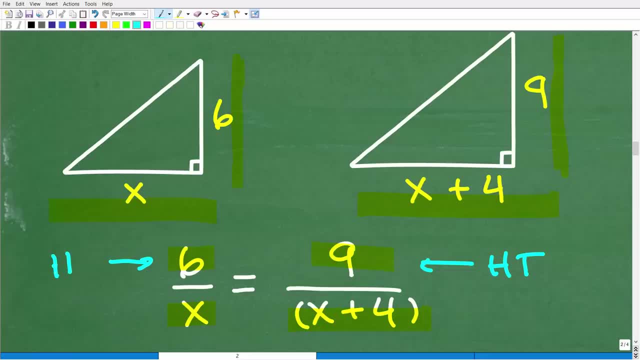 careful here that we're talking about the height of these triangles. Okay, that is our numerators, and then the length is our denominators, but they are in proportion. So, in other words, this ratio is equal to this ratio and we can set up what we call a proportion, which is two equal ratios. So here is 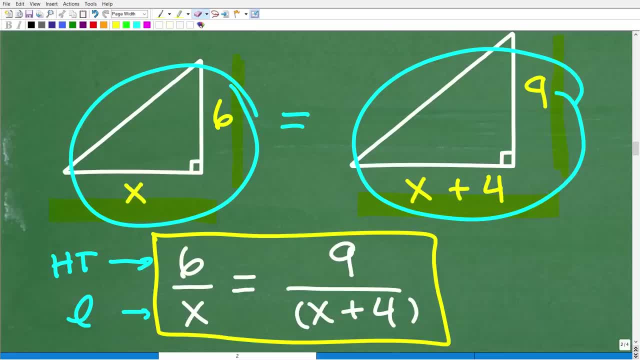 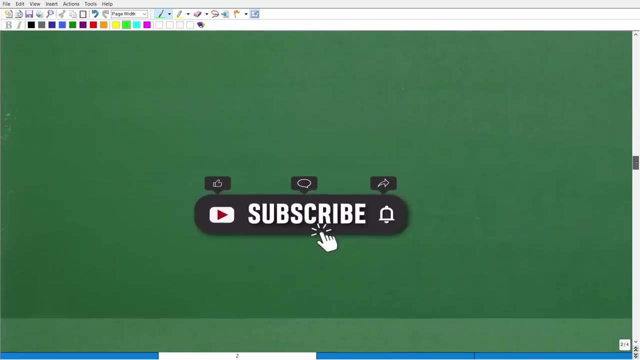 the key to figuring out the problem. Alright, so we have a proportion: six is to X, as nine is to X plus four. So now really comes down to your ability to solve this equation, Alright, so let's go ahead and do that right now, but before we do that, I need you to do this, and that is to hit that subscribe. 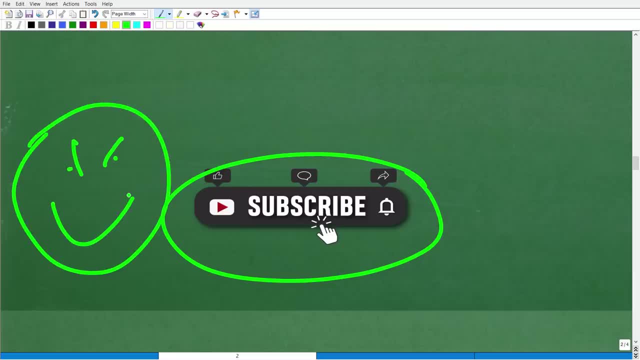 button. You see, I got to kind of sneak that in because I definitely need your help to continue to grow my YouTube channel so I can help as many people as possible. You see, for me as a math teacher, I'm happiest when I'm teaching mathematics and I'm really truly. 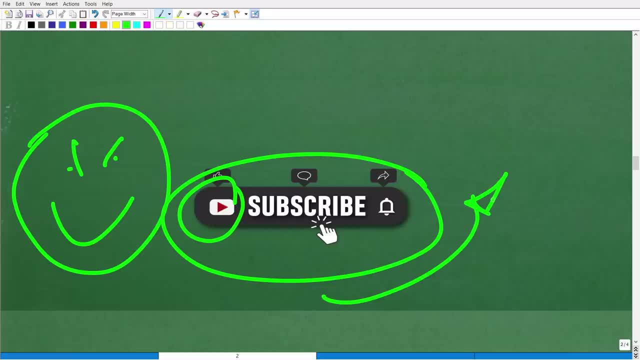 you know, happiest when I'm helping people learn math and the more people I can help, the better. you know. you know I feel about myself and you know these problems. I try to make math interesting. you know I don't like to just do kind of like standard math problems. Now, this is kind of a 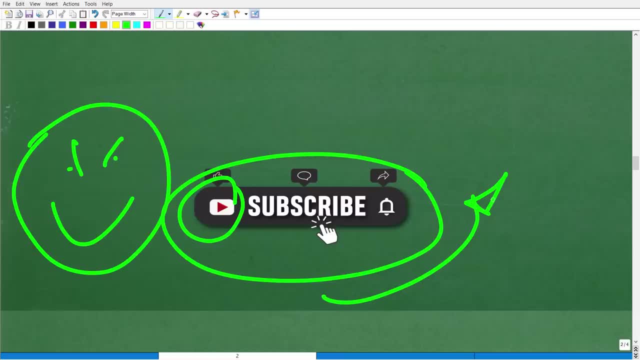 typical math problem but I try to, you know, teach it in a way that people like and understand and, importantly, I try to give a lot of people out there that are struggling in math encouragement to not give up. So if you need help in mathematics, check out my full main math courses. you can find 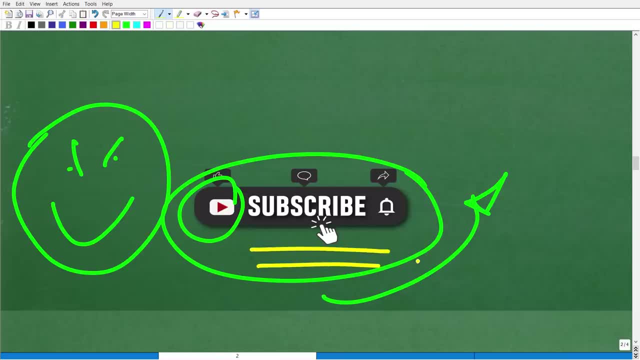 links to those in the description of this video. and if you want to know more about similarity, congruency, kind of the geometry topics that we're talking about here, two recommendations. one: you can check out my full geometry course- you'll find the link to it in the description- or my math skills. 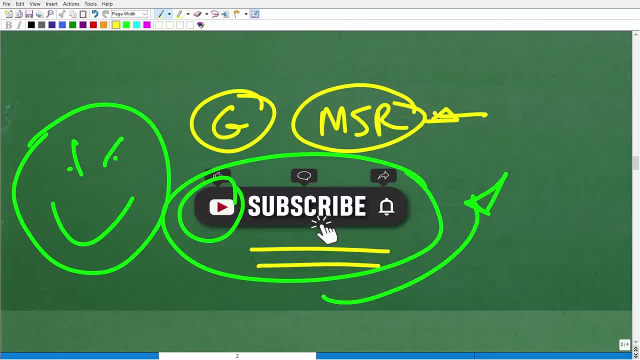 course you that have been away from math and you want to kind of relearn math, starting from the basics, and this course I go through basic arithmetic, algebra, a ton of geometry and even some basic trigonometry and probability and statistics. Okay, so let's go ahead and figure out this. 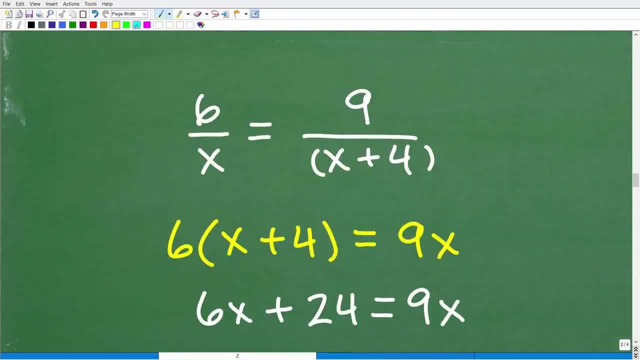 proportion, and what we need to do here is use something called the cross product. this is how you solve proportions. So we have one fraction that's equal to another fraction, so this is, by definition, a proportion, So we can cross, multiply this way. this is called the cross product. so when you have a proportion, 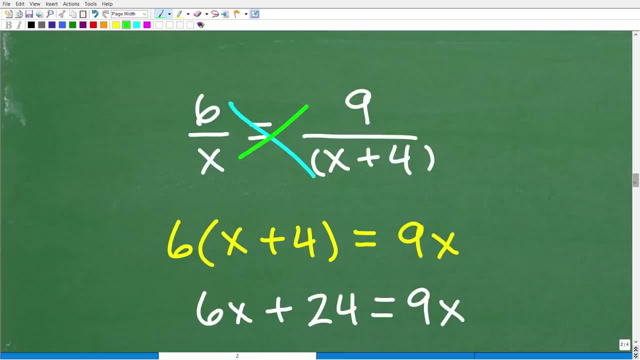 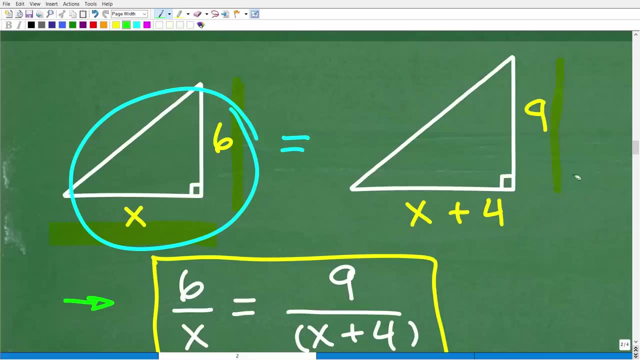 the cross products are equal. Now, one thing you have to be super careful about here is when we set up the proportion. notice in this triangle, the larger triangle, that the length is X plus 4. but anytime you have a sum or difference, you want to put parentheses around it. oftentimes you won't. 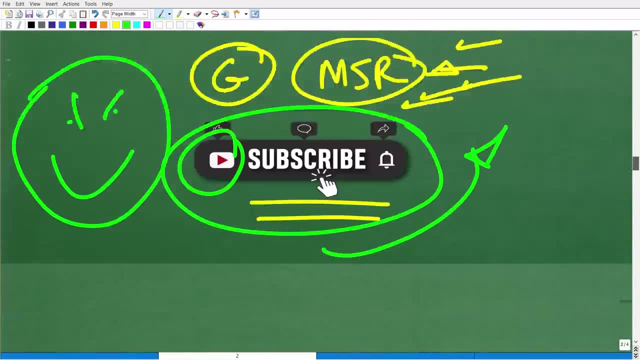 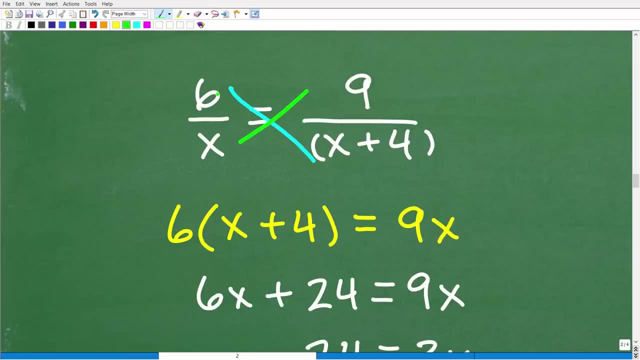 have the parentheses, so put those in, because if you don't, you can easily make an error. All right, so we have parentheses around our X plus 4, so now we're going to go ahead and cross multiply. so this is going to be 6 times X plus 4, so we're going to write it just like this. 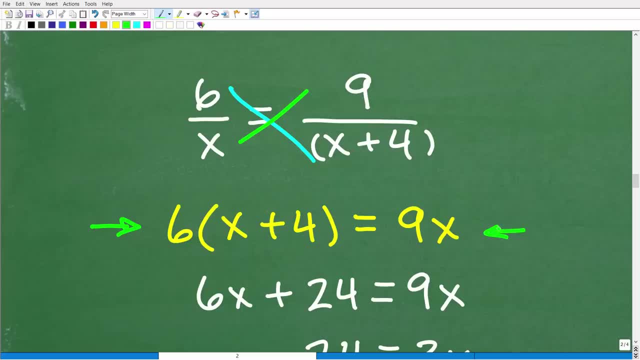 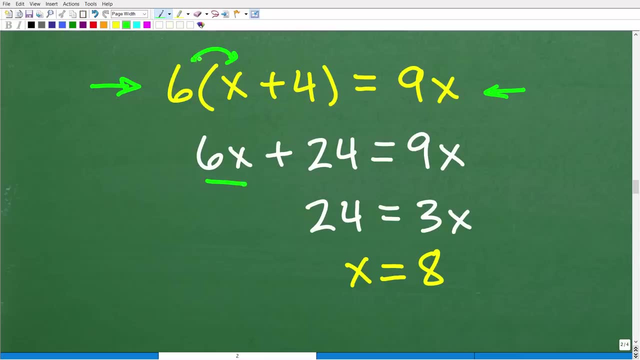 with the parentheses, and then 9 times X is 9 X. Okay, so we cleared the fractions. now we just need to go ahead and do the algebra. so this is going to be 6 times X or 6 X, and then 6 times 4 is 24. 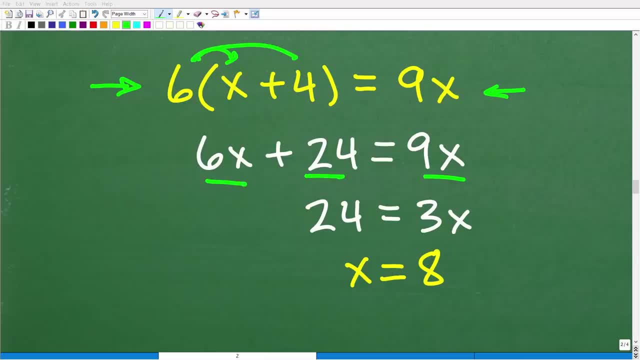 and that's equal to 9: X. So now let's go ahead and move our variables to one side of the equation and our numbers to the other side. Now, typically, we like to put our variables on the left and our numbers on the right, something like. 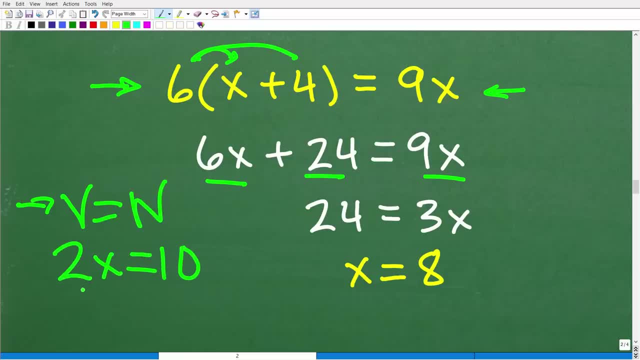 say 2 X is equal to 10, but you could also have: 10 is equal to 2 X if it's easier to take a step. so, in other words, in this particular situation, if I wanted to move my variable terms to the left, I'd 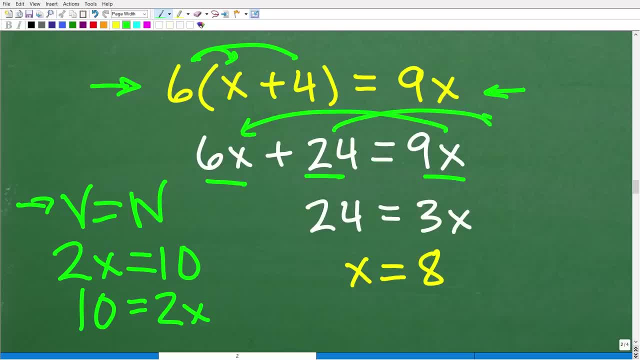 have to move the 9 X over here, but then I'm going to have to move the number to the other side. so that is two steps. but to make my life easier I could just simply go. you know, what I'm going to do is I'm just going to keep my variables on the right, so all I have to do is subtract 6 X from